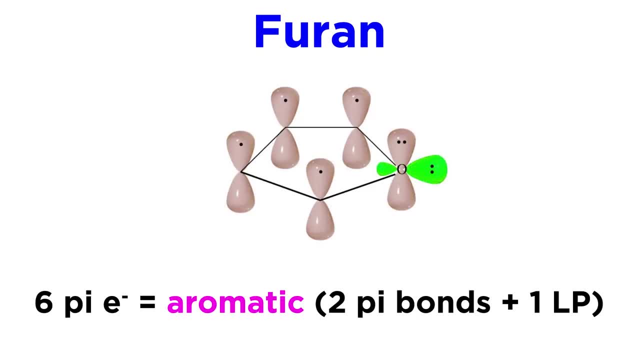 with one oxygen atom and two pi bonds. We must understand that furan is aromatic, given that one of oxygen's lone pairs is part of the pi system, allowing it to be fully conjugated, and there is a total of six pi electrons which satisfy the number of atoms in the ring. 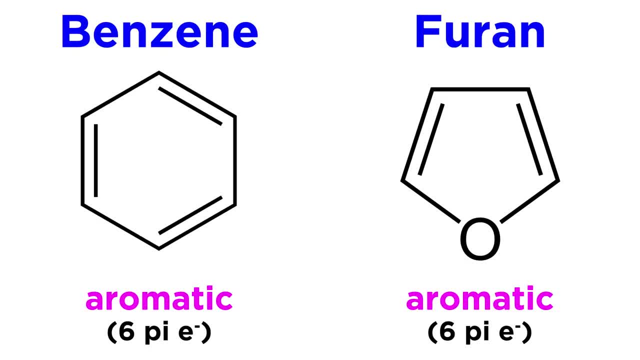 So it's a little bit like benzene, just with an oxygen in there, though it is actually quite a bit more reactive than benzene, given that its delocalization energy, or resonance energy, is only 16 kcal per mole, compared to benzene's 36 kcal per mole. Let's also note the numbering. 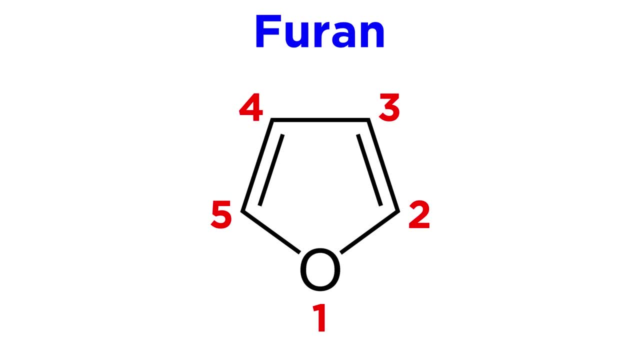 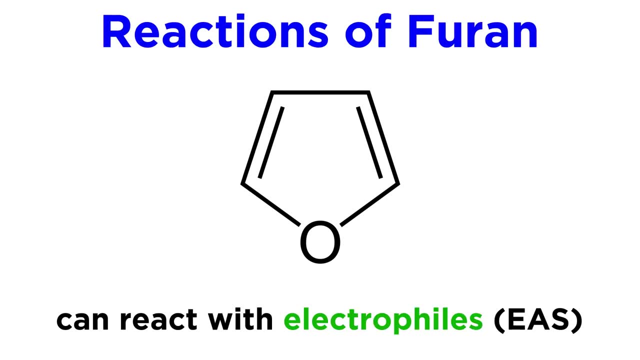 system which always labels the oxygen atom as number one, and going around in either direction from there. So what does furan do? Furan will react readily with electrophiles in ways that resemble the electrophilic aromatic substitution reactions we've learned, simply without the necessity. 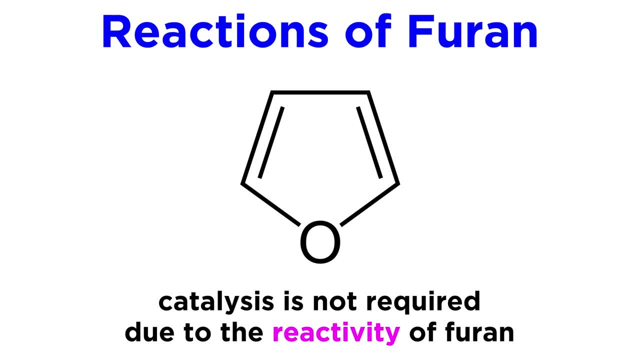 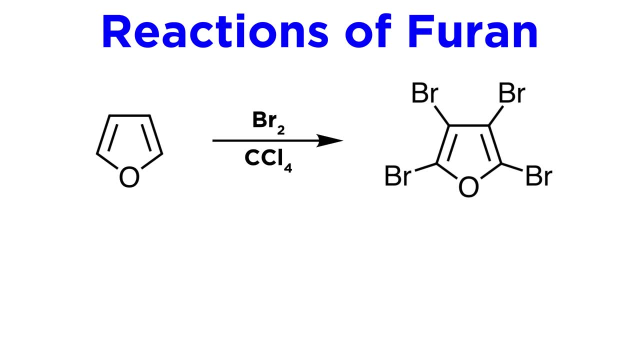 for a catalyst, since furan is more reactive than benzene, For example. furan will react with bromine in carbon tetrachloride, and it will do so at a rate that is hard to control, which tends to result in tetrabromofuran. Friedel-Craft's reactions can also. 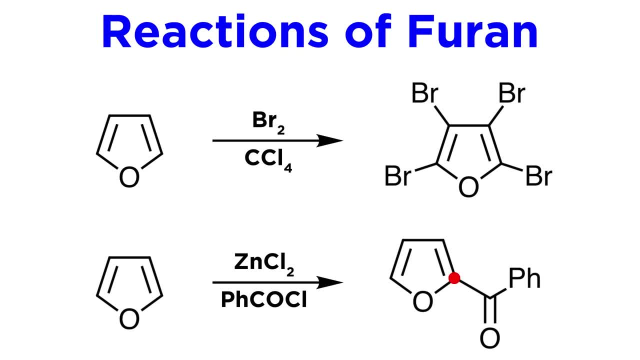 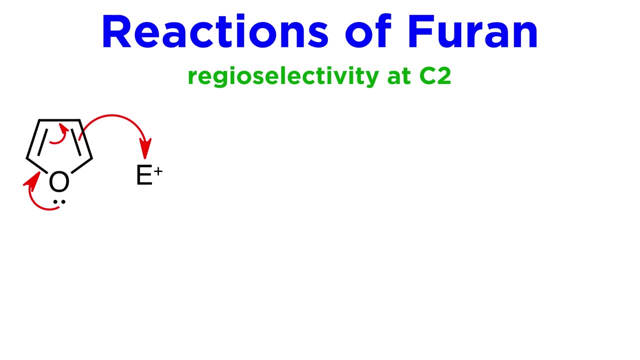 be performed, and these are a bit more selective, occurring primarily at carbon 2.. This Friedel-Craft's acylation is an example of this kind of chemistry. The regioselectivity here can be explained as follows: If we push a lone pair from oxygen around the ring to pick up the electrophile, we are left. 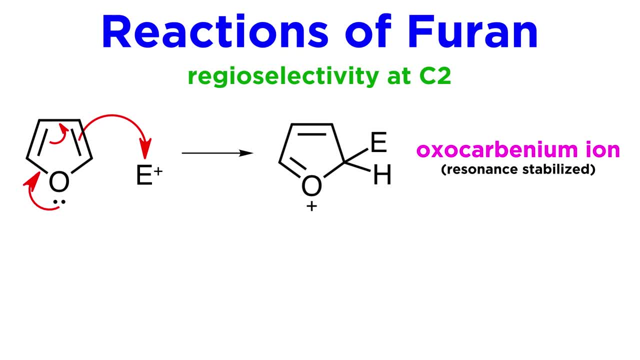 with a conjugated cationic species called an oxocarbenium ion. This would not occur if the electrophile ended up on carbon 3.. This would not occur if the electrophile ended up on carbon 3.. So resonance is the primary factor guiding the regioselectivity here. 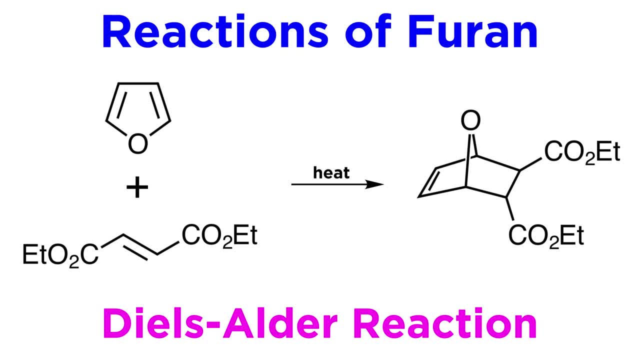 Furan can also act as a diene in a Diels-Alder reaction and, because it is electron-rich, it can easily react with any activated dienophile, such as diethyl fumarate, even under moderate conditions involving slight heating to generate the product we see here. 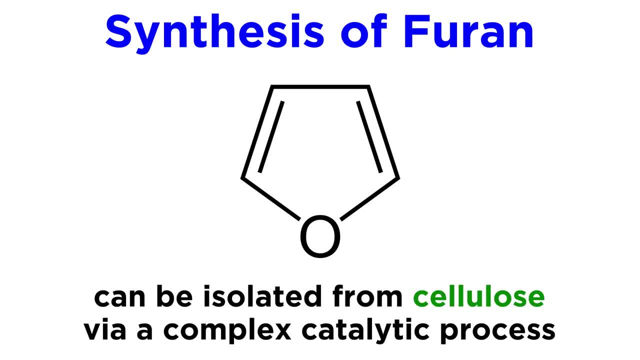 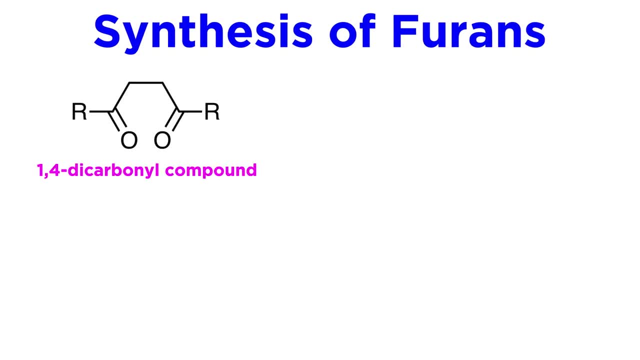 To quickly cover how furans are formed. it is possible to isolate furan from cellulose via a complex catalytic process, but more interesting is the synthesis of substituted furans from 1,4-dicarbonyl compounds. This occurs via acid. 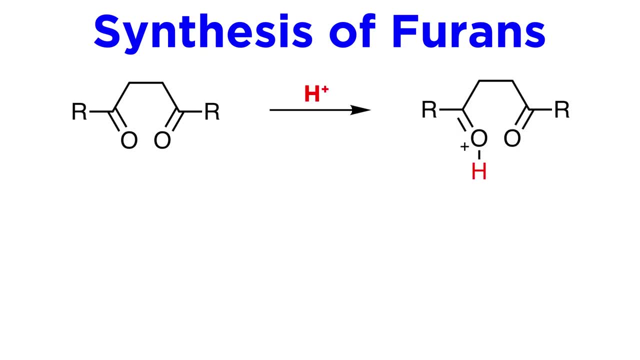 catalyzed dehydrative cyclization. As you can see, one carbonyl is protonated, which prompts attack from the other carbonyl oxygen. After further protonation, elimination of off water and the elimination of another proton neutralizes this oxygen atom, leaving us with a. 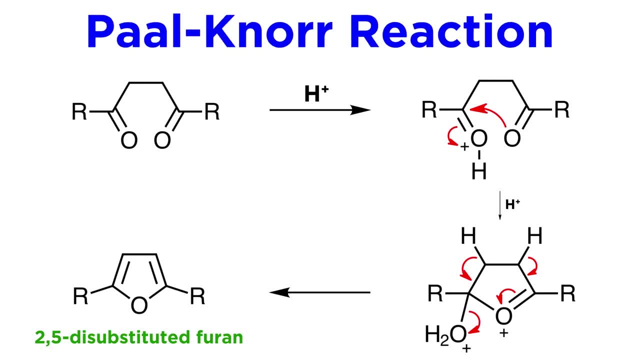 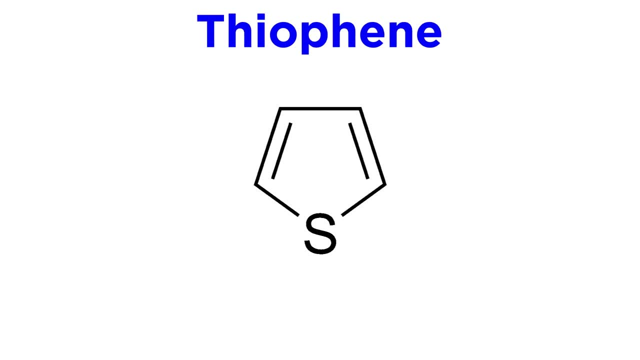 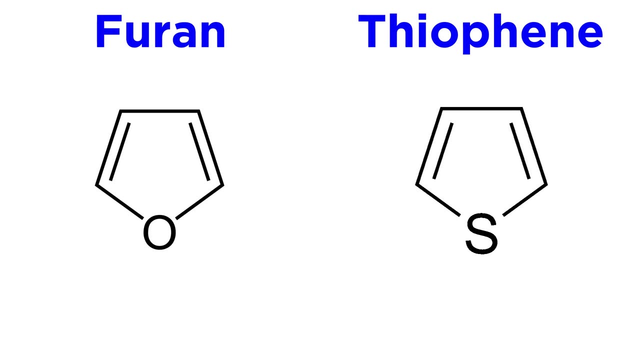 disubstituted furan. This process is known as the PAL-NOR reaction. Now let's move on to thiophene. This is the sulfurous analog of furan, in that the molecule is almost the same, just with a sulfur atom instead of oxygen, However, its resonance energy 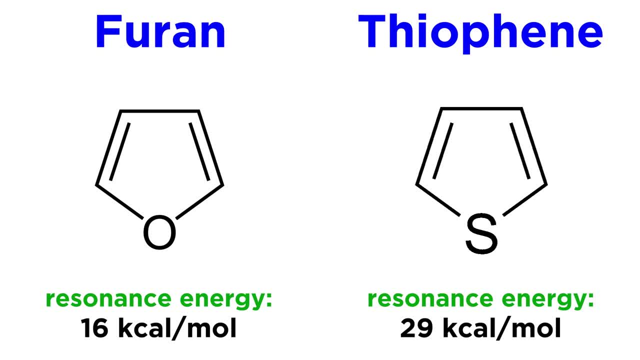 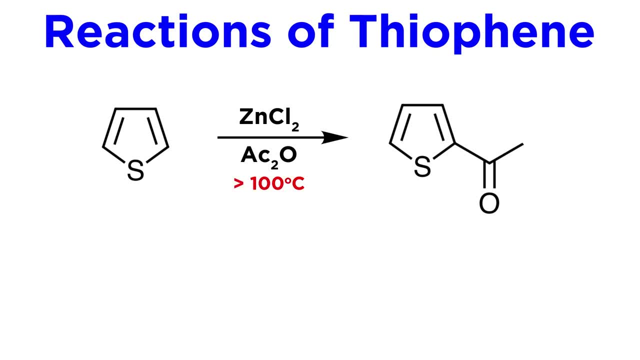 is 29 kcal per mole, so it is quite a bit less reactive than furan, For example. looking at the same Friedel-Crafts chemistry we examined earlier, much higher temperatures are required to carry out the reaction on the thiophene substrate. In addition, thiophenes are not reactive enough. 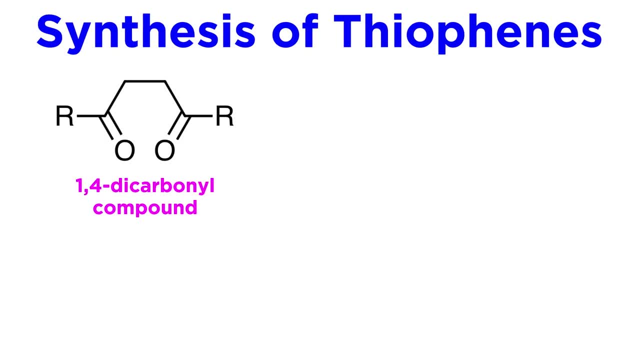 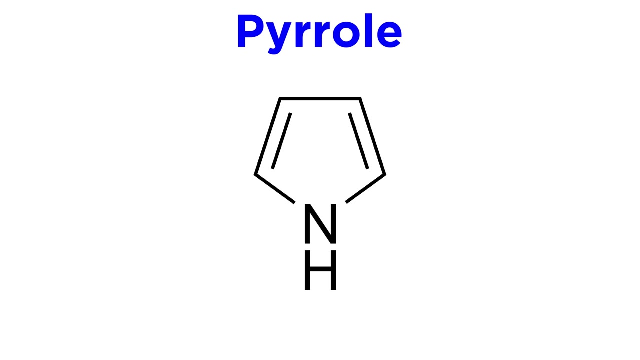 to participate in Diels-Alder reactions. Interestingly, they are prepared identically to the technique we learned a moment ago with furans, starting with a 1,4-dicarbonyl compound. Finally, we have pyrrole, which is again similar to furan, just with a nitrogen atom instead of. 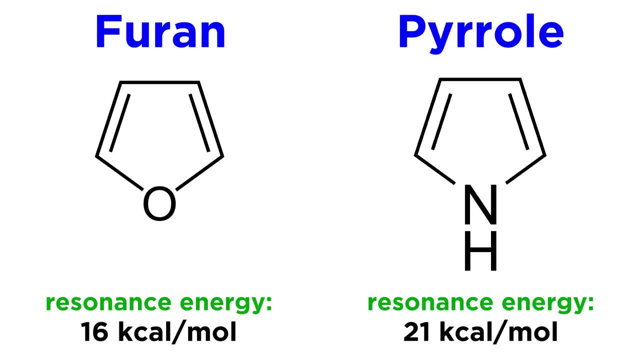 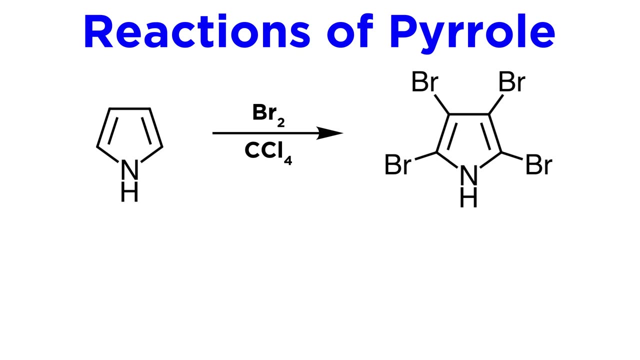 oxygen, which is bound to a hydrogen atom With a resonance energy of 21 kcal per mole. its reactivity is similar to that of furan, typically reacting at carbon too. For example, pyrrole tetrabrominates easily, making the monobromination product difficult to attain even at low temperatures. 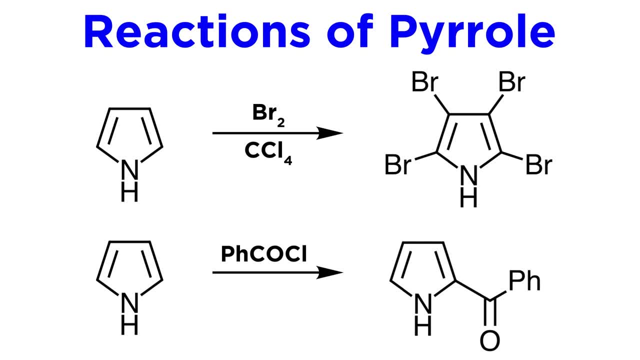 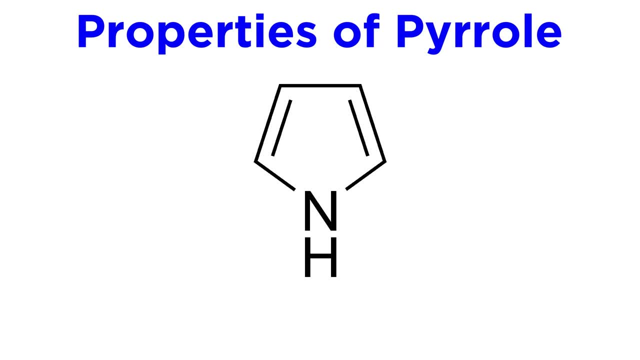 Also like furan Friedel-Crafts. acylation happens easily, even without lewis acid activation. An interesting feature of pyrrole is that, despite the nitrogen atom, it is not basic. In fact, if protonated by a very strong hydrogen atom, it will not be able to activate the pyrrole. However.